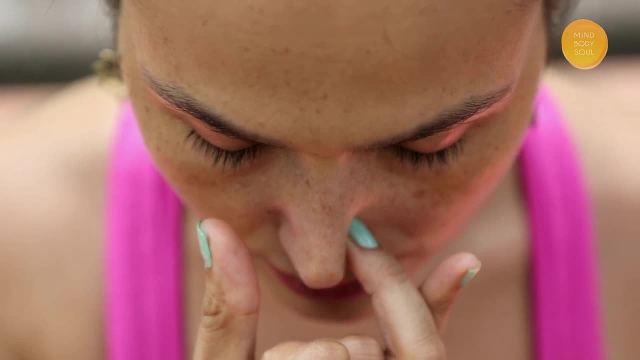 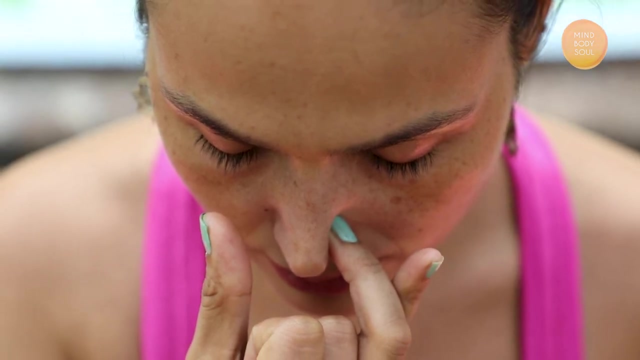 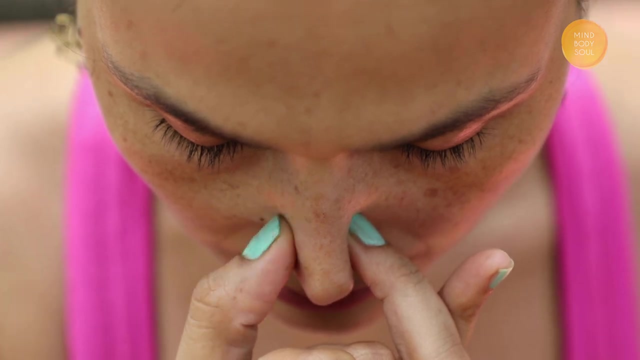 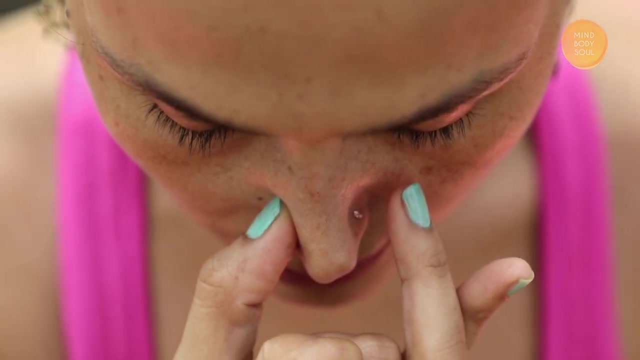 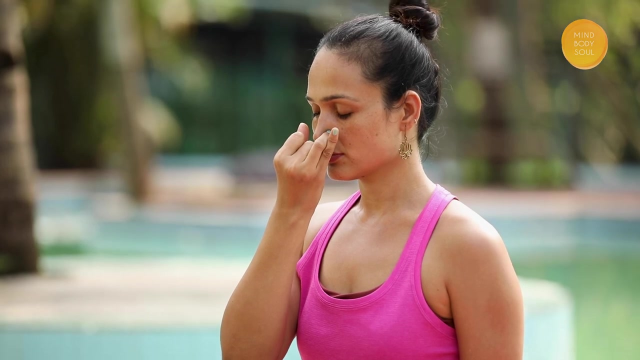 and simultaneously exhaling through my right nostril as I release my thumb from there. I'm again inhaling through my right nostril and closing the right nostril, and exhaling through the left as I release my ring finger from there. I have completed one round of anulom vilom here You. 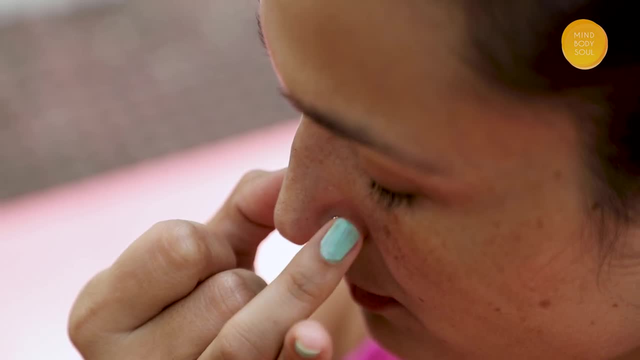 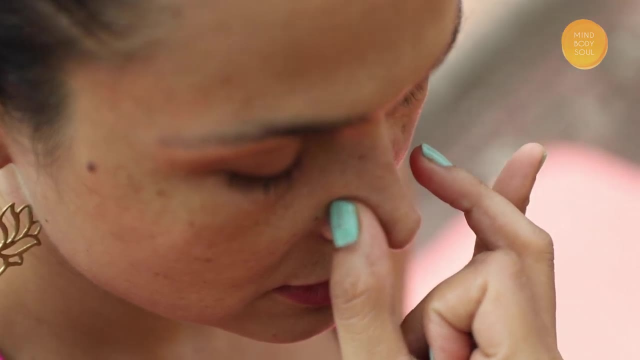 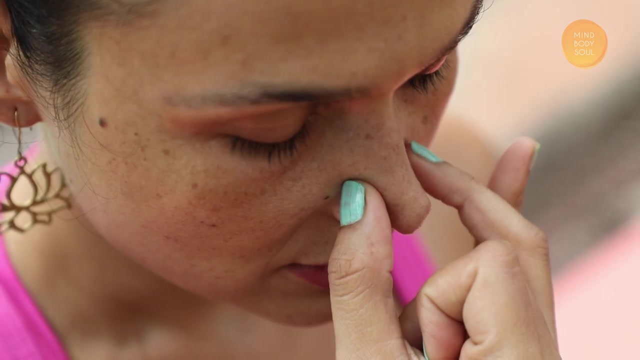 can repeat the same cycle of breathing for 5 to 15 rounds All throughout the practice. try to keep the inhalation and exhalation equal as much as possible. If you are a beginner, start with one minute and then gradually extend to five minutes. 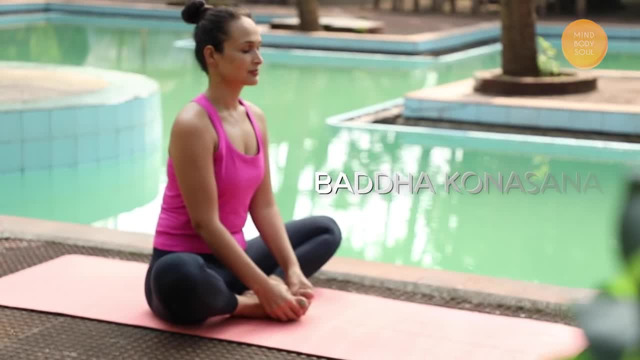 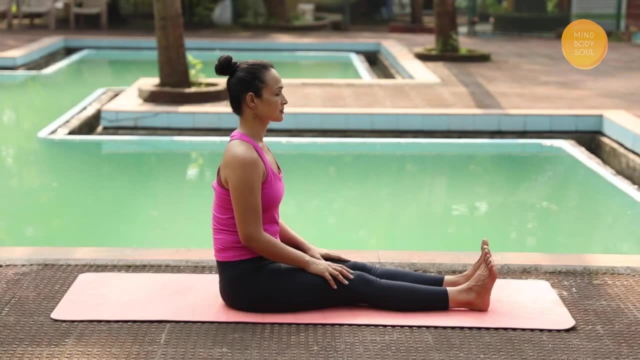 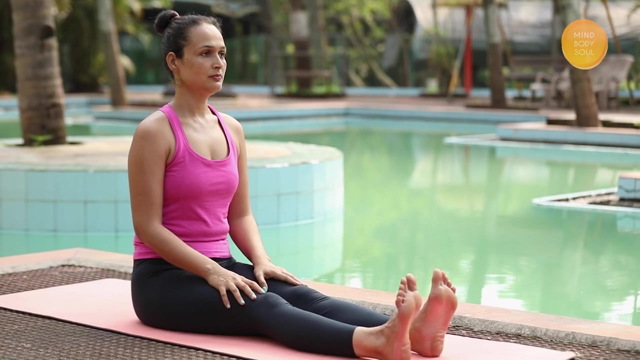 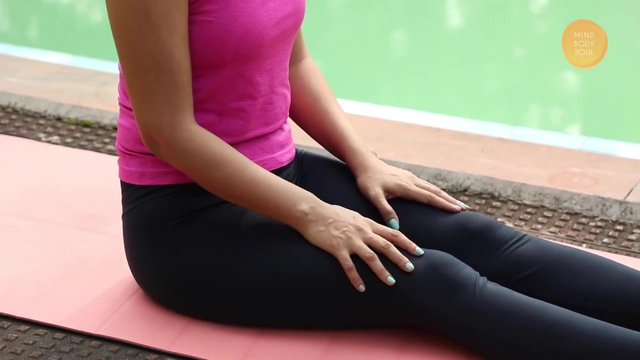 The first pose which I am performing is called baddha konasana, or the butterfly pose. I'm beginning this pose by sitting with my legs extended straight and spine lengthened. Sit on your sit bones as much as possible. I'm keeping my arms relaxed with my palms on my thighs. We have 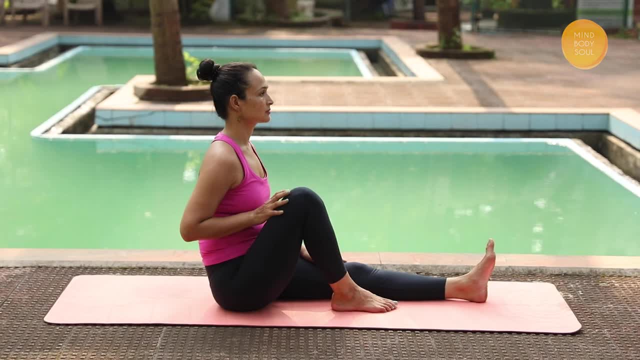 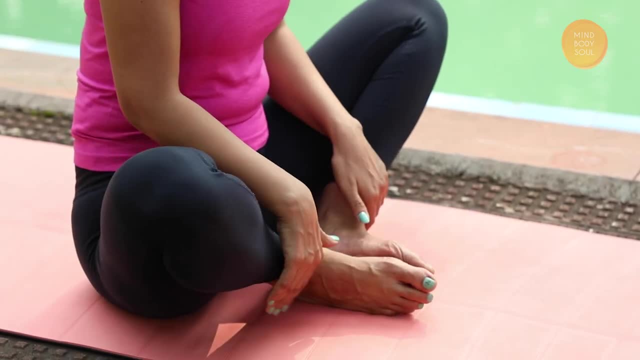 to keep breathing normally throughout. Now I'm bending both my knees, one by one, and bringing the soles of my feet together. While exhaling, bend the knees. I'm bringing the soles together. Now I'm bringing the soles of my feet together. While exhaling, bend the knees. I'm bringing the. 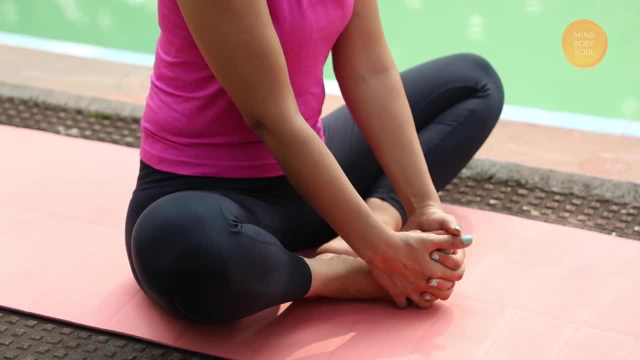 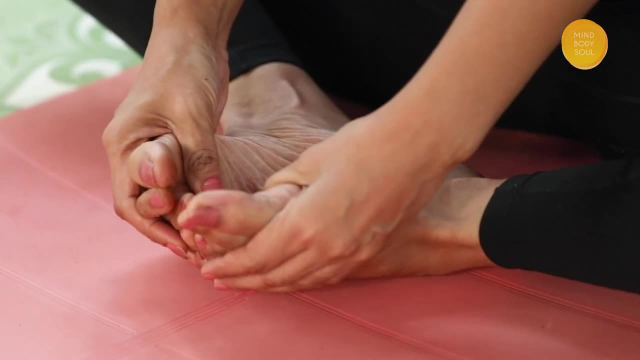 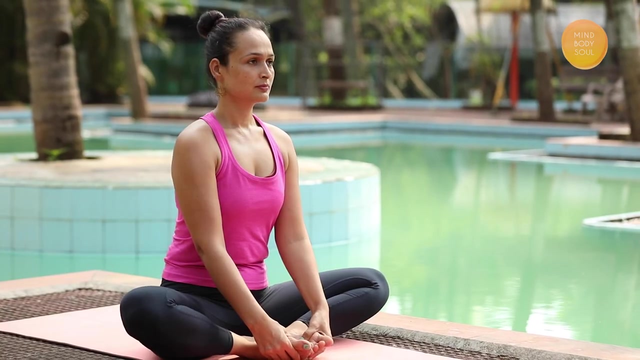 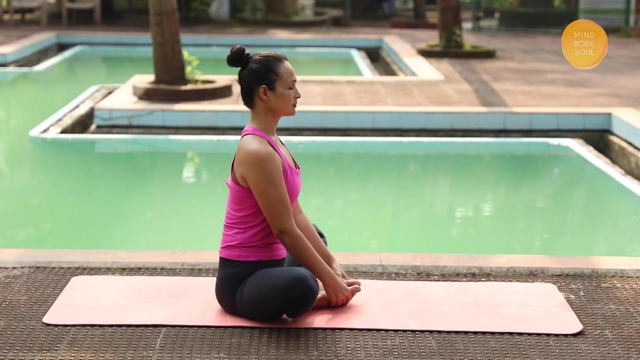 while I let my knees fall out on the other side, I'm drawing the soles of my feet together and using my hands to open them, as if opening the pages of a book. I am taking a deep breath, stretching my spine upwards and exhaling slowly. 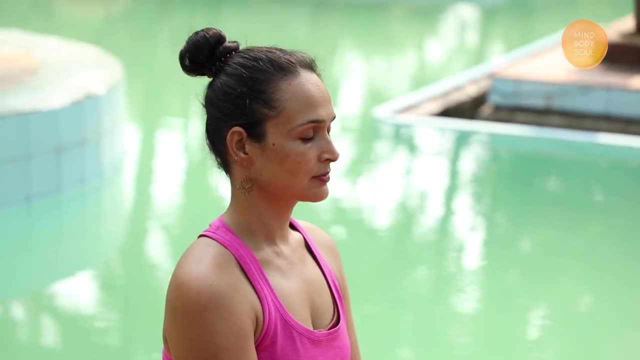 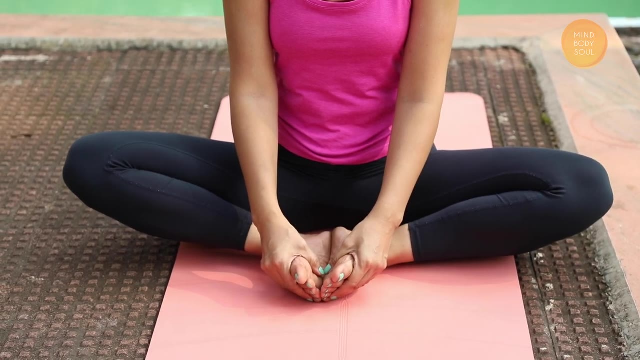 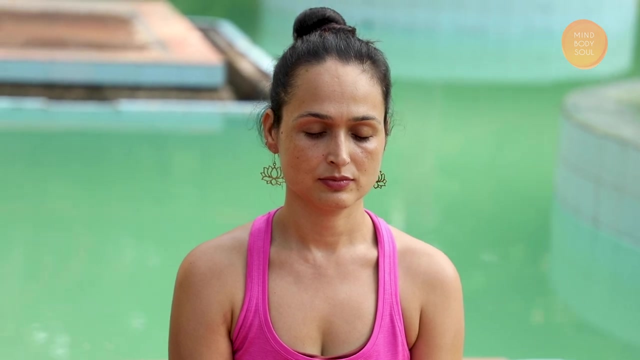 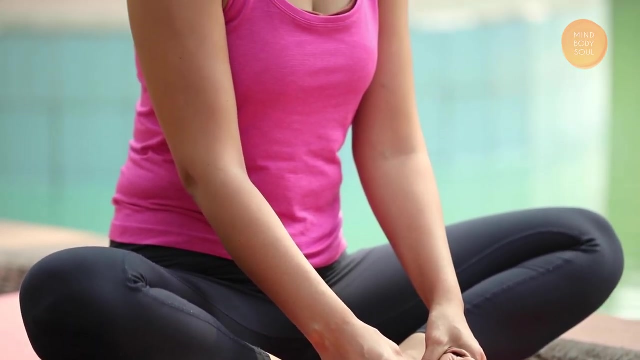 I am making sure that my shoulders and arms are relaxed. I can feel the inner thighs stretching, the lower abdomen and the back relaxing. With my eyes closed, I am observing my breathing for 3 to 5 repetitions. If you are not comfortable sitting on the floor, 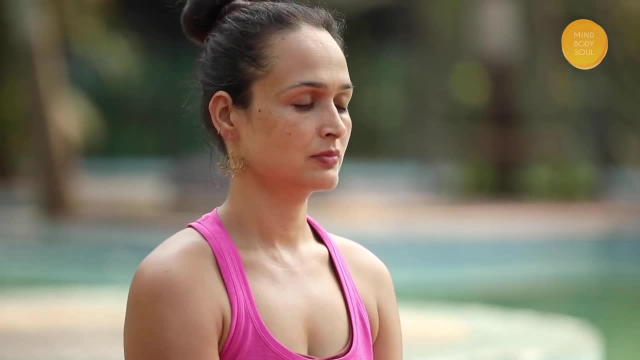 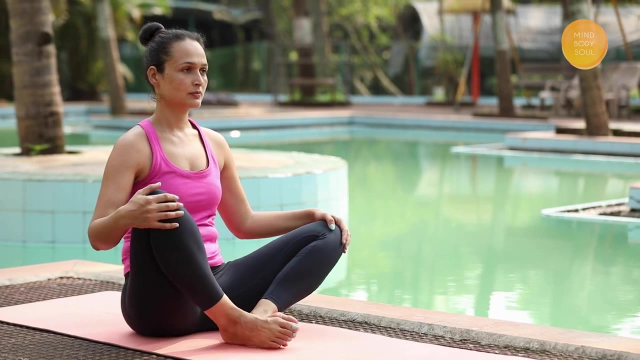 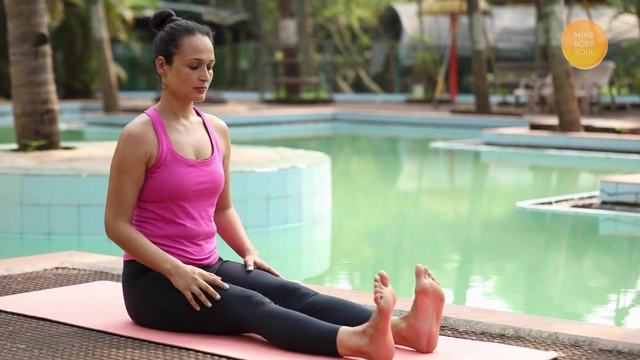 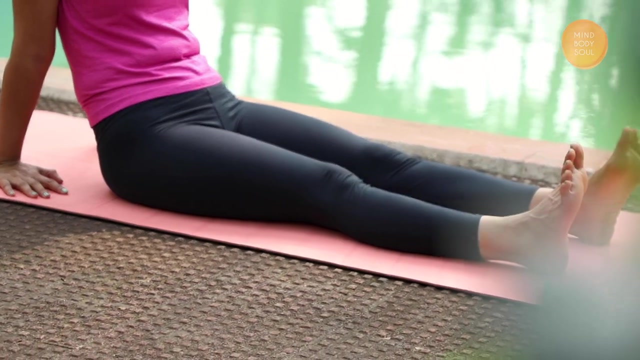 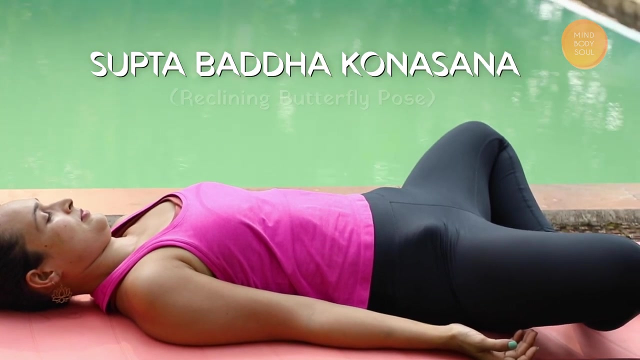 you can use a cushion too, To release my pose. I am gently opening my eyes, relaxing my arms and straightening my legs. The third asana is called Supta Baddha Konasana, or the Reclining Butterfly Pose. 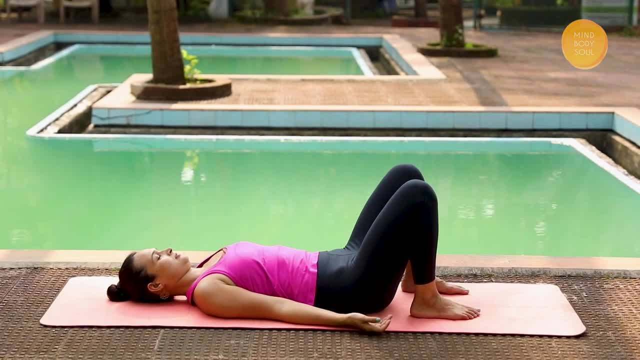 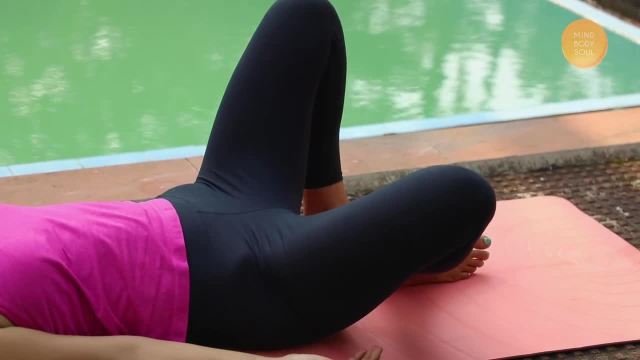 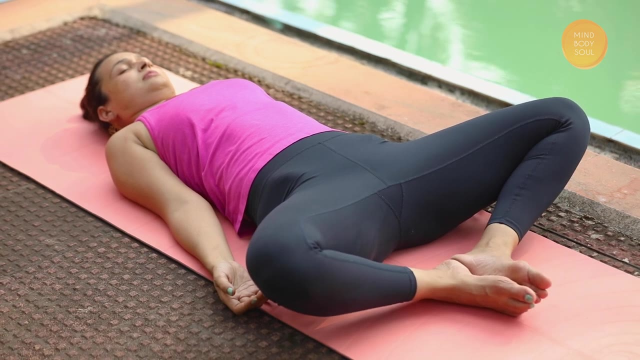 I am lying on my back with my knees bent, keeping the soles of my feet on the floor. Next, I am opening my knees on either side, bringing the soles of my feet together. I am keeping my legs in the same position. 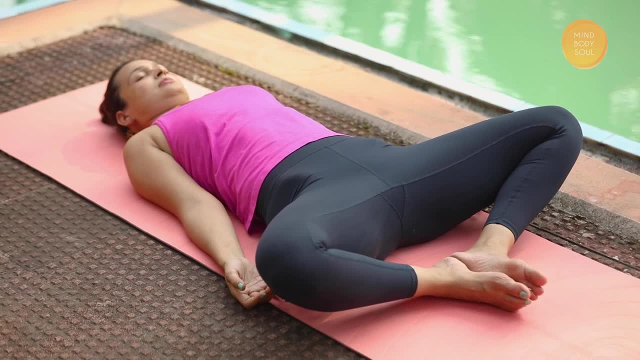 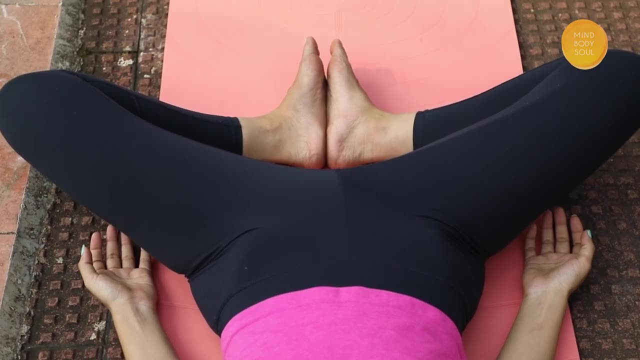 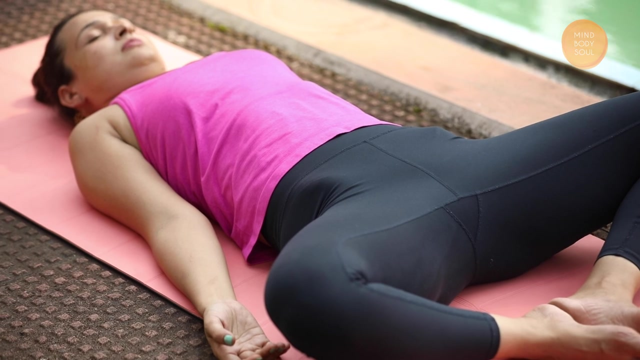 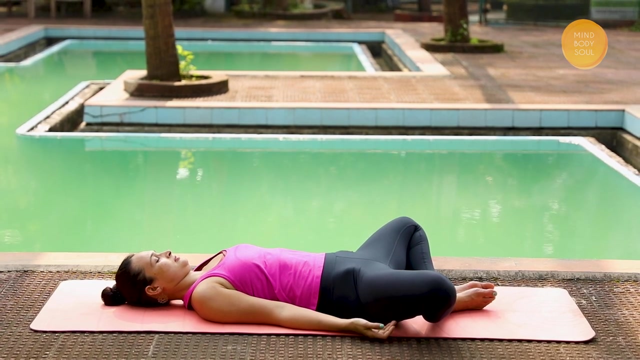 as they were in Baddha Konasana. My arms are relaxed by my side. I will be staying here for several minutes as gravity works to deepen my stretch. I am breathing naturally throughout my pose, While in this pose focus on relaxing the back and pelvic area. 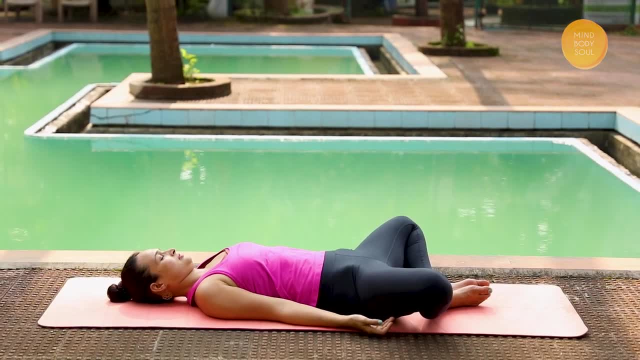 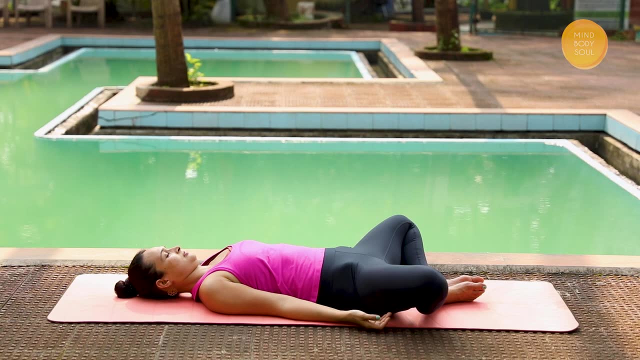 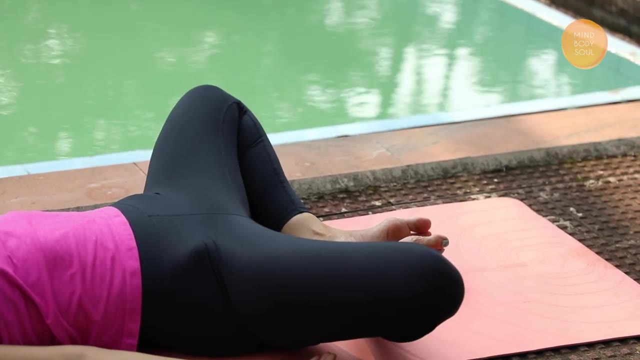 Take longer and deeper breaths, which will surely make you feel better. As you exhale, keep your hands on the floor. As you exhale, keep your arms and legs on the floor. Make sure you don't push your knees towards the floor. 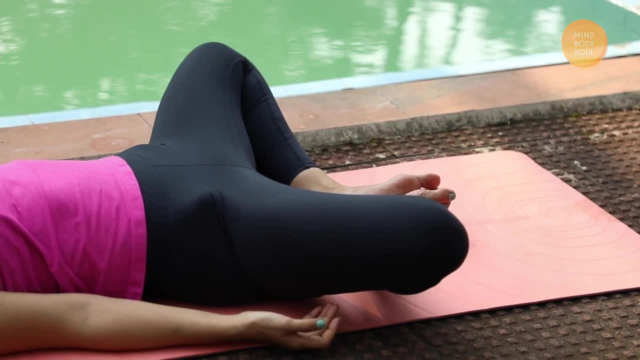 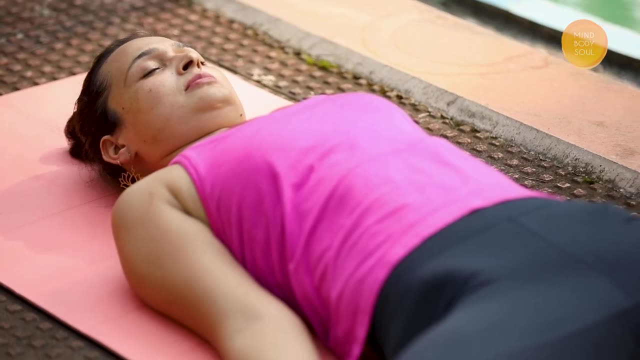 Rather than gravity. let your hip joint and thigh muscle release this tension gradually In case you are facing lower back pain or knee injury. please avoid this pose. You can hold this pose for as long as you are comfortable, When you are feeling anxious. 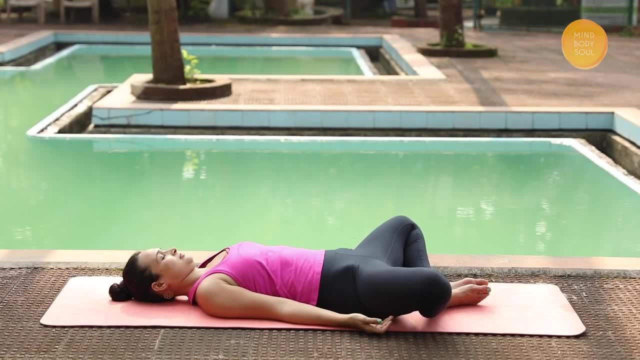 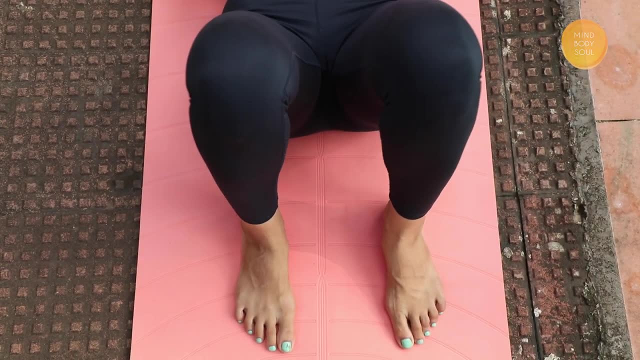 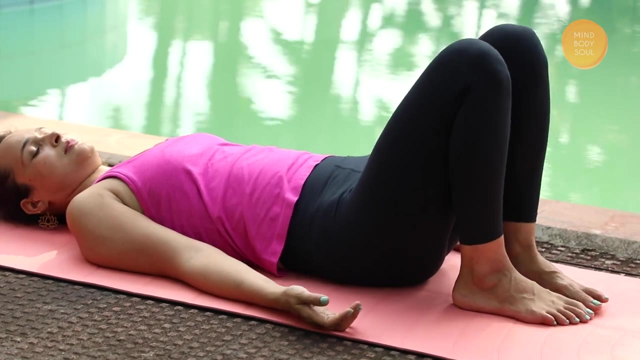 or you feel like you are losing your balance. please give a few kisses If you are feeling tired When you want to conclude. come back to the initial position, where the knees were bent and feet were on the floor. I am rolling over to one side and using my hands to support as I sit up. 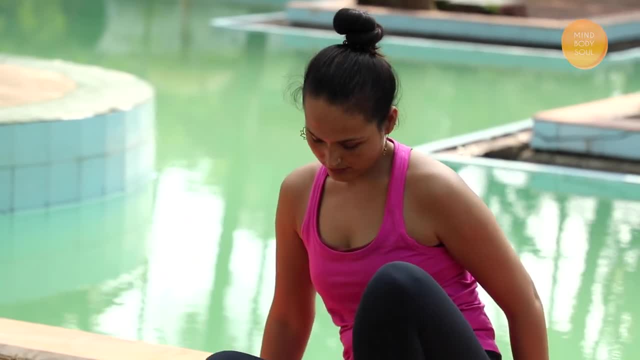 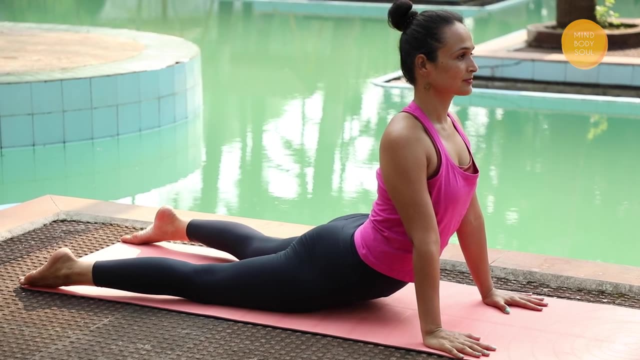 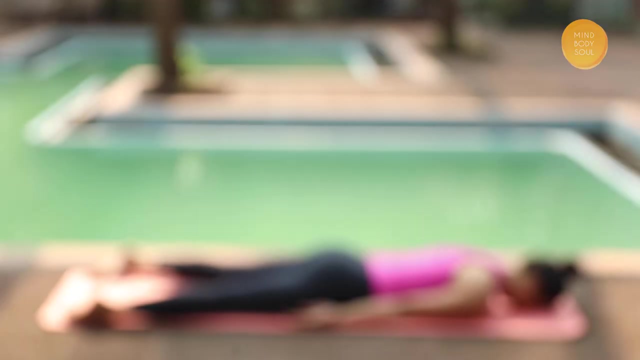 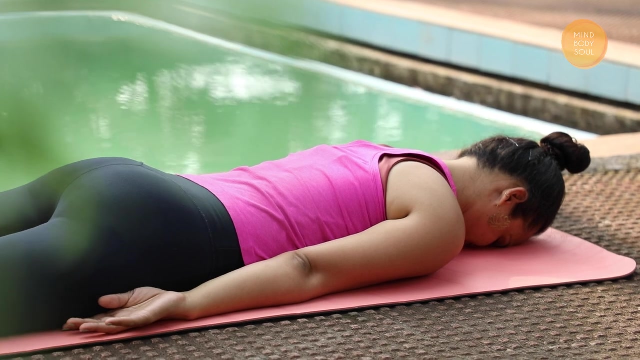 The fourth and final pose I am performing is called Bhujangasana, or the Cobra pose. I am beginning this pose by lying on my chest with my elbows close to my body and palms facing up. As I am inhaling, I am moving my arms to the side. 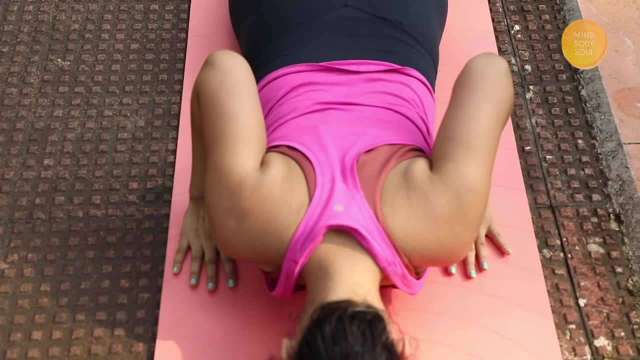 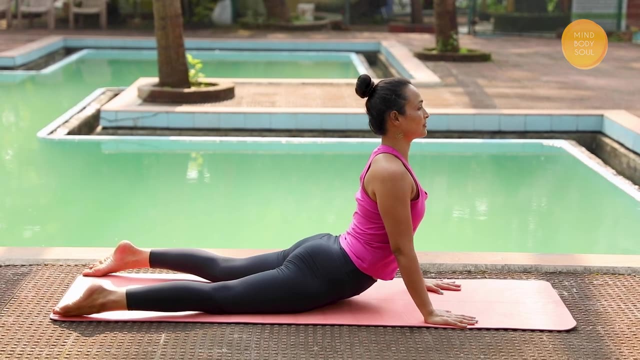 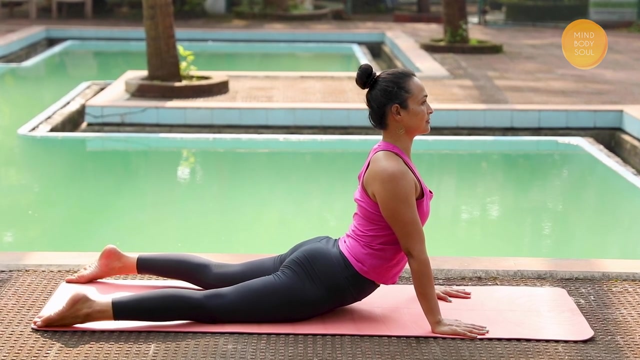 As I am inhaling, I am slowly straightening my arms to lift my chest off the floor and keep reclining my back. I could notice a beautiful stretch when I lifted my chest. I am keeping my gaze forward. You can even keep it up if your neck is comfortable. 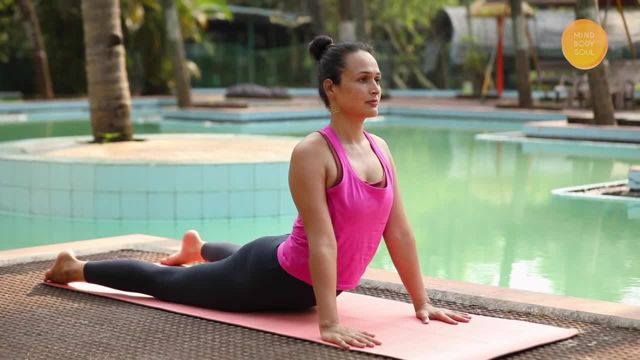 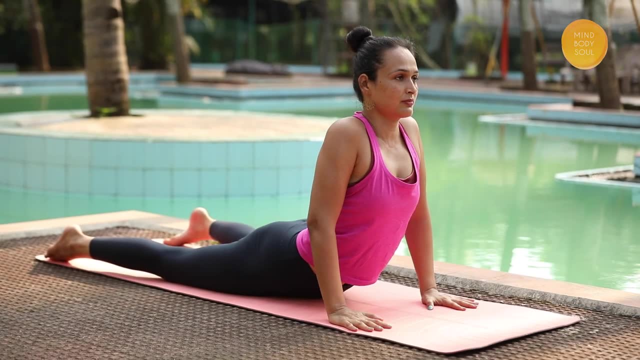 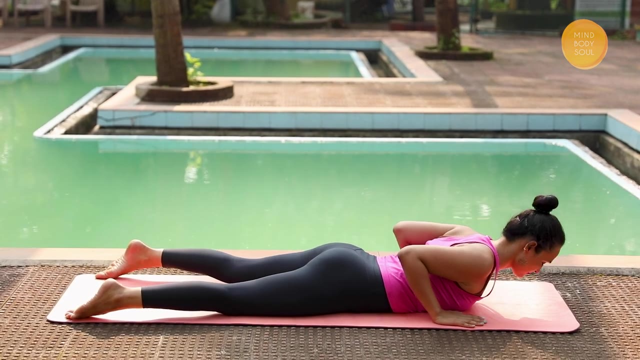 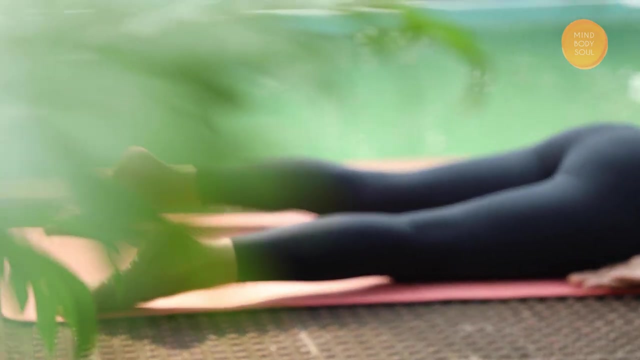 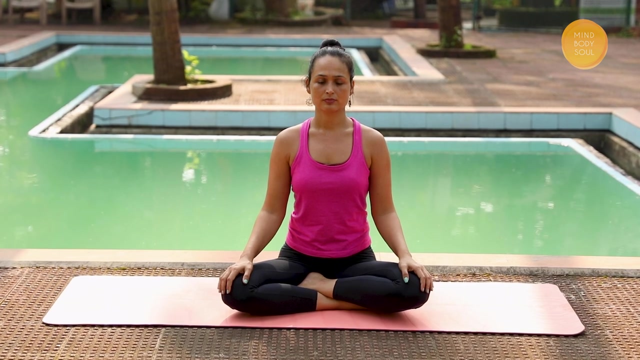 I am holding this posture for 15 to 30 seconds. If your shoulders crunch during the pose, bend both your elbows and lift your chest higher, Gradually exhaling. I am returning to my normal posture. Let's finish our session with a calming breathing practice called Brahmari Pranayama or the Bumble Bee Breath. 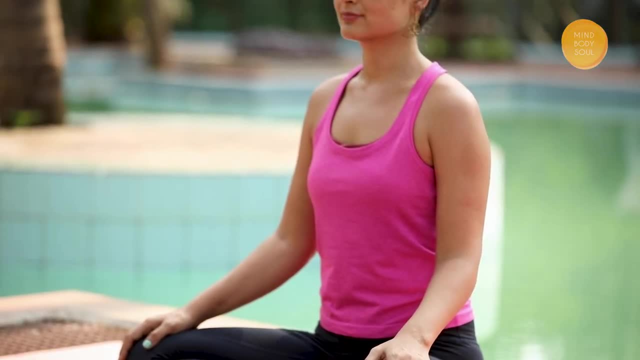 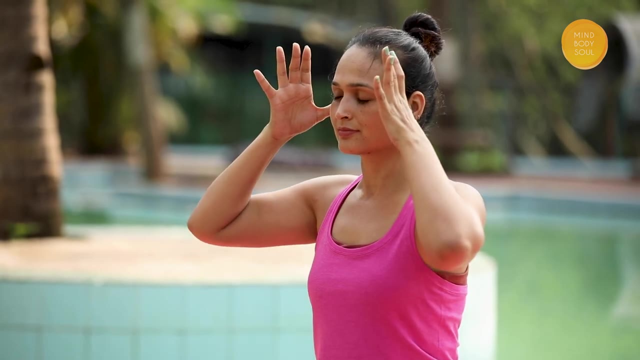 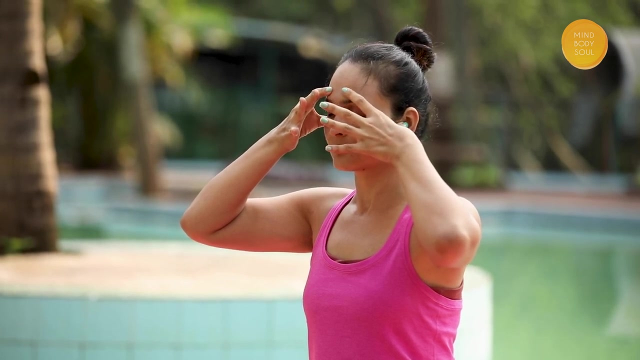 I am sitting in Sukhasana. I am closing my eyes and taking deep breaths. I am closing my ear flaps with my thumbs. I am placing my index finger just above my eyebrows and the rest of my fingers are covering my eyes. 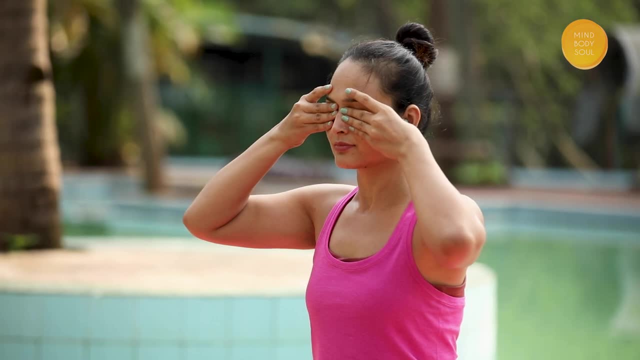 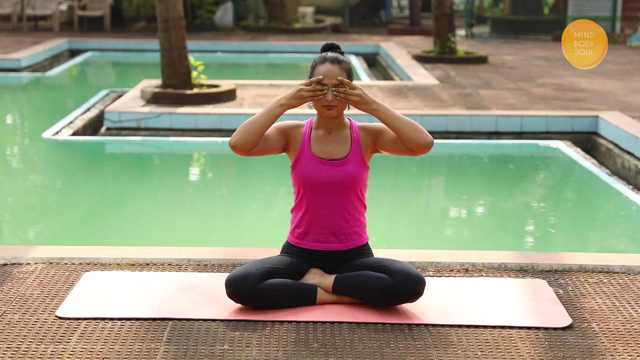 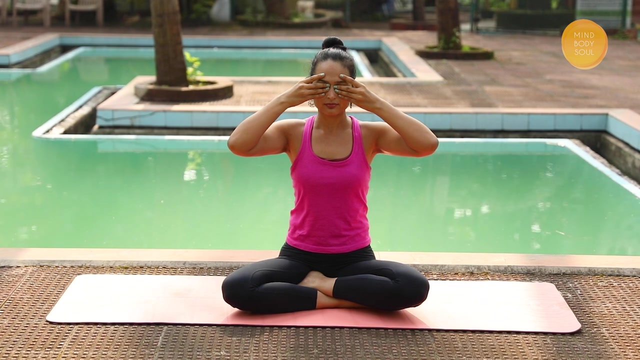 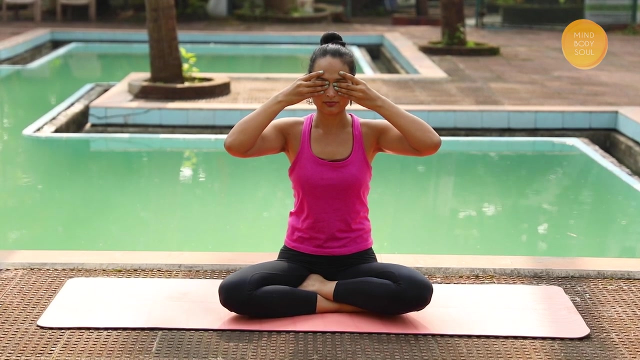 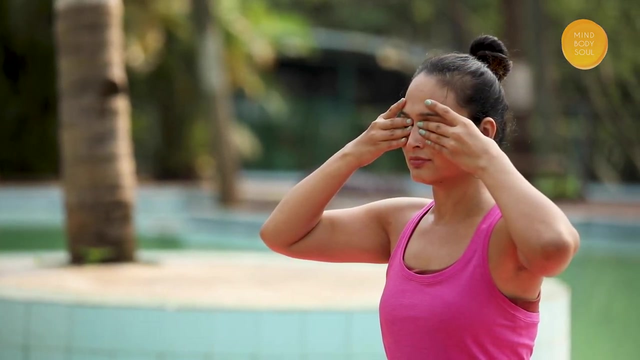 Now I am applying gentle pressure on the sides of my nose, I am concentrating my mind on the area below, I am keeping my mouth closed and I am breathing out slowly while humming the sound of. For better results, repeat this five times. The important thing is that, while doing this, Pranayama.